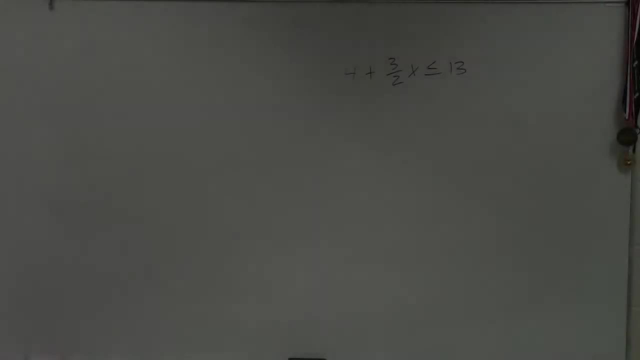 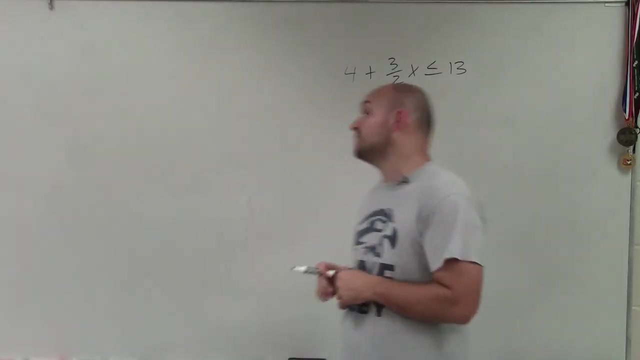 Welcome, ladies and gentlemen. So what I'd like to do is show you how to go ahead and solve this absolute value. not absolute value, just this inequality. So in solving inequalities, just like solving equations, except we're going to have to graph our solutions. We don't. 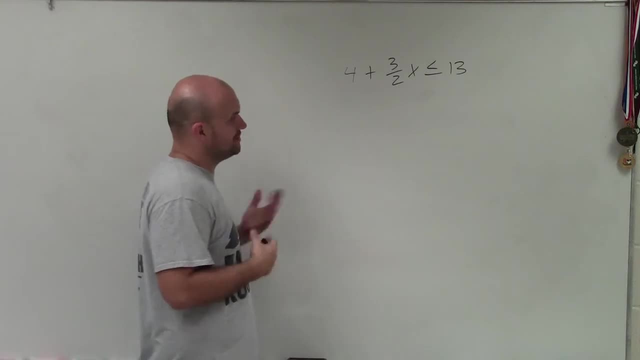 have to, but that's the way we like to represent our solutions with a graph. Now we have a fraction. People don't like fractions, So I'm going to show you two different ways to be able to solve this. So the first way is just using our inverse operations. 4 plus. 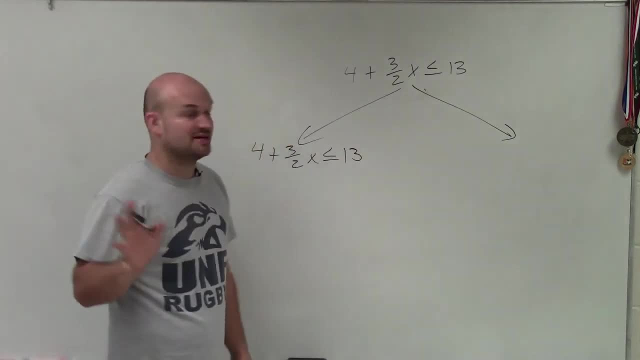 3 halves x is less than or equal to 13.. And I'll make it very quick, I swear So, to solve this using my inverse operations. just first thing I have to do is undo addition and subtraction. So I have 3 halves x is less than or equal to 9.. Now to go ahead and solve this now. 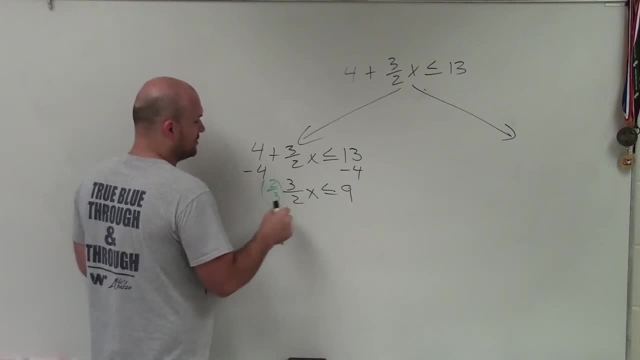 I've got to get rid of my fraction. I can just multiply by the reciprocal. And to get rid of fractions, just always think: multiply by the reciprocal. So any time you take a fraction and multiply it by its reciprocal, it's going to go to. 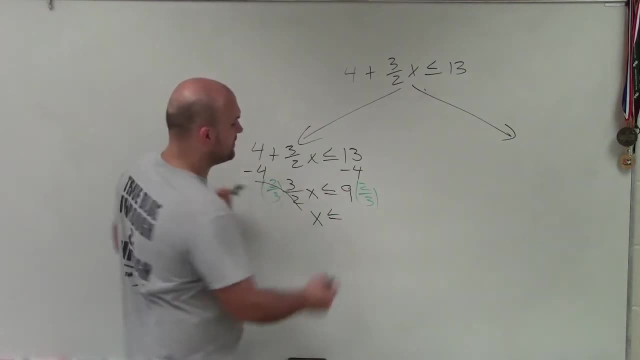 1.. So x is now less than or equal to 9 times 2 thirds. Just multiply across, That's really 9 over 1.. So 9 times 2 is 18.. 18 divided by 3 is going to be 6.. x is less than or equal. 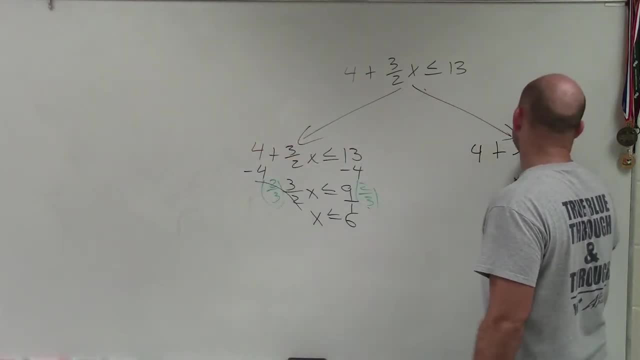 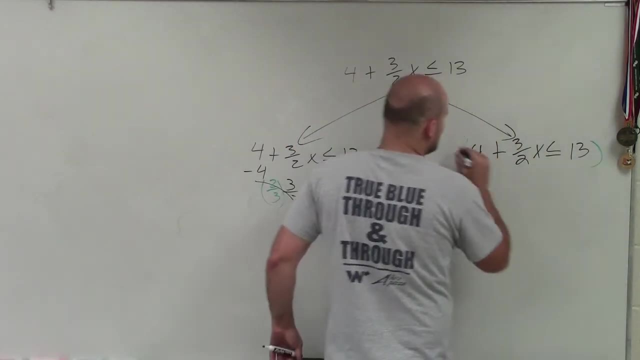 to 6.. Now I'll be very brief with this, But a lot of times, students, they have trouble with fractions. Just get rid of the fractions. Multiply everything by 2.. If you multiply everything by 2, you're creating an equivalent inequality. 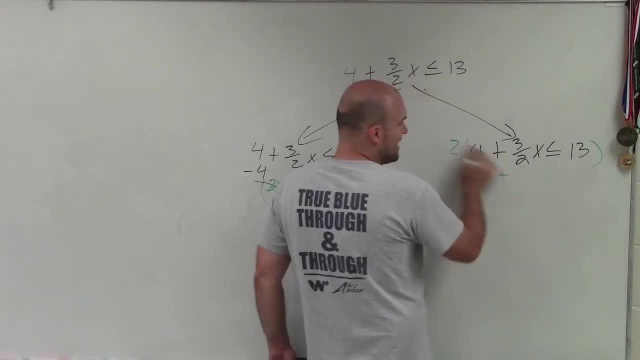 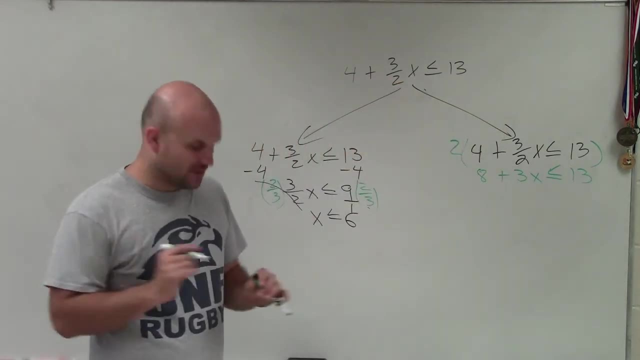 So you have 8 plus Now 2's. divide out, So it's 3x less than or equal to 13.. From there, if you go and solve, you'll get 6. I swear. So anyways, we know x is less than or equal. 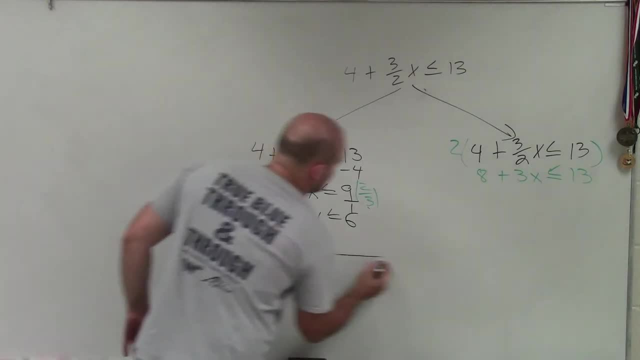 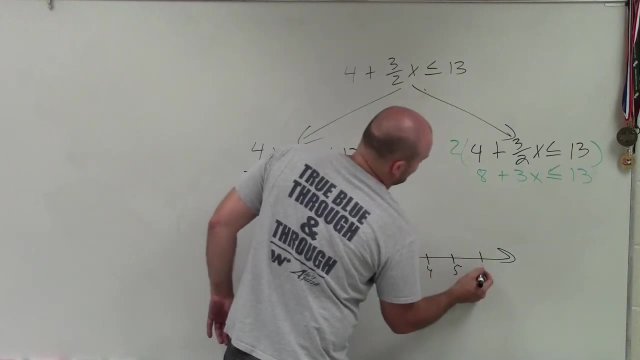 to 6.. Let's go ahead and graph that. So have an inequality of 0,, 1,, 2,, 3,, 4,, 5,, 6, 7.. OK, So now we go to 6. And we make a nice big dot, And then we need to use our 3. So we 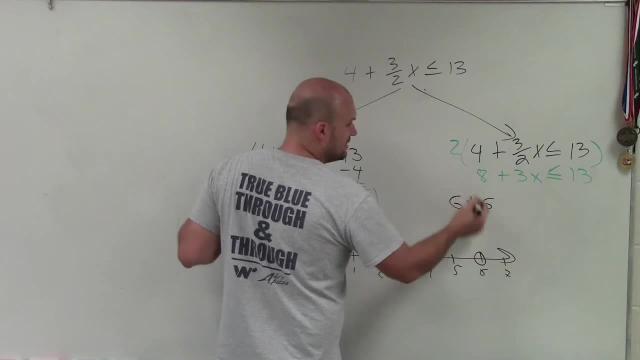 test points. So we test 6.. Is 6 less than or equal to 6?? Yes, that is true. So, since it's true, this 6 is a part of our solution. So we fill it in, Then we just pick points.